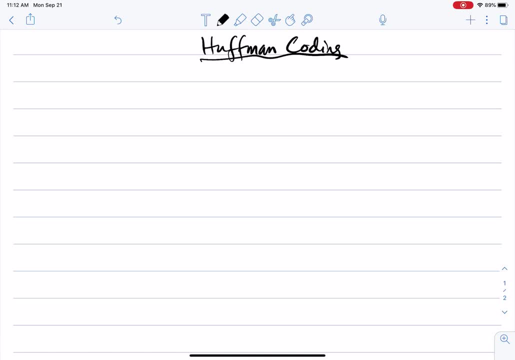 imagine that we have a string W, or let's string W here, let's say here: we have a string W here, let's say here, whose length is say 100, 145 million characters. okay, hundred forty five million letters, and the letters are either a or B or C or D. okay, you get a. 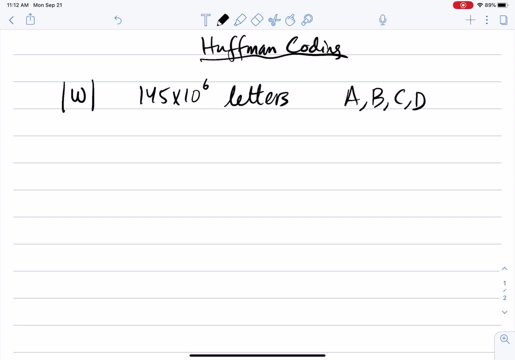 very, very long string of ABCD's and D's, and our job, our task, is to turn W into binary representation. so represent W as a binary string. what does it mean to represent W as a binary string? we need to find what. what this means is find 4. 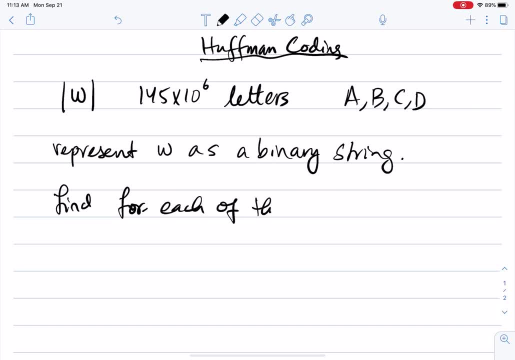 each of the four letters, the four letters ABCD, binary code words and use these code words to represent W. okay, so we need, for example, to find a equals some, you know, binary string B is another binary string, and so on. now the objective function here. objective function, what is it that we are trying? 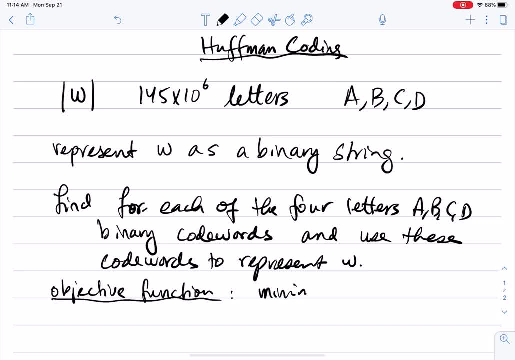 to optimize. we want to minimize the length of the binary encoding of W. okay, so let us make this more concrete, maybe with a few, with an example, okay, so again, remember, someone gives me a long string. in this case I'm trying to say other string is four letters ABCD, if 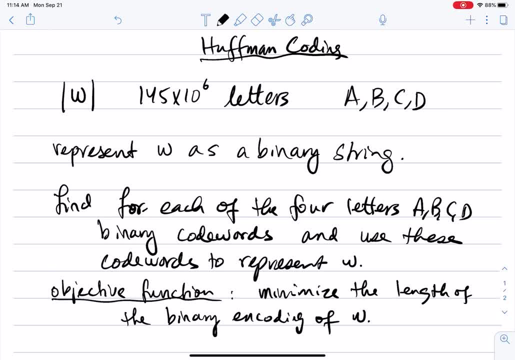 this is DNA, a CTG. and someone gives me a genomic sequence that has 144 million nucleotides in it. every nucleotide is a letter, a CTG. they want me to compress it by first turning it into a binary string of zeros and ones, and 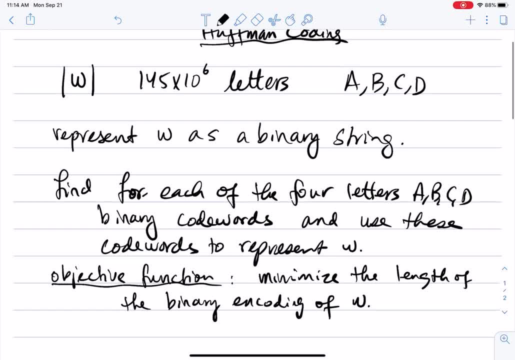 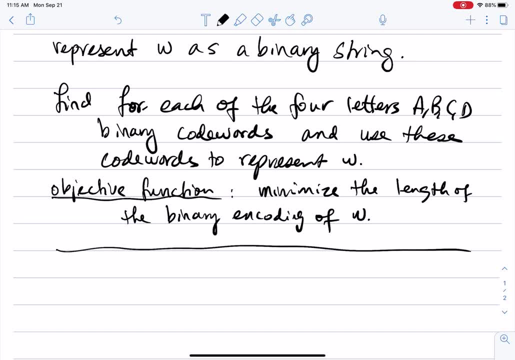 but they want that string of zeros and ones to be the smallest possible. so we have 145 million. okay, so one possible solution, one solution. first solution is: let us actually encode a as a zero zero, B as zero one, C as one zero, D as one one, since there are four letters. 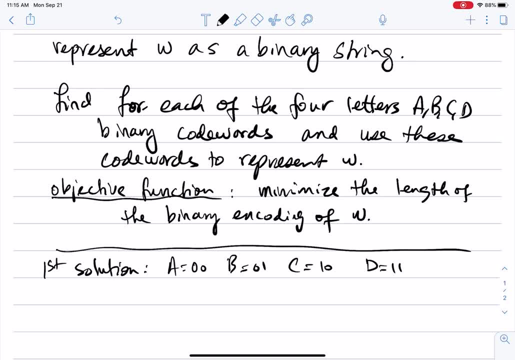 we need two bits to represent all of them in four different code words. right, so we have zero, zero, zero, one, one, zero one one. so now, what will becomes the length of the encoded, of the encoded string? well, the string itself was 145 million, and each one of these let 145 million letters, and each one of these letters now. 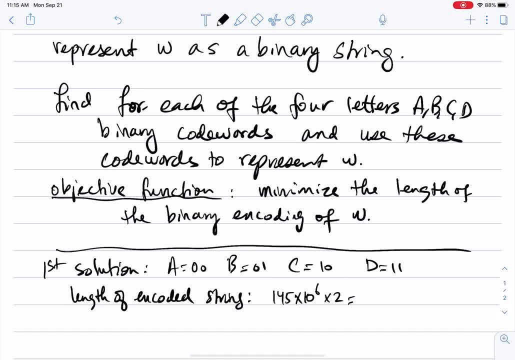 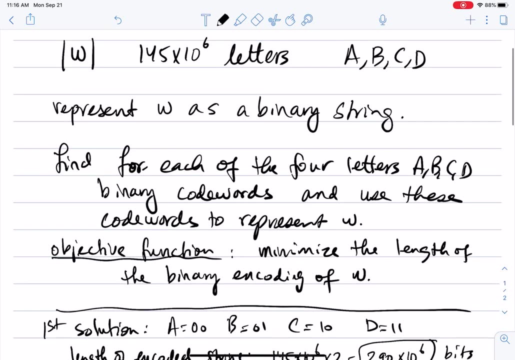 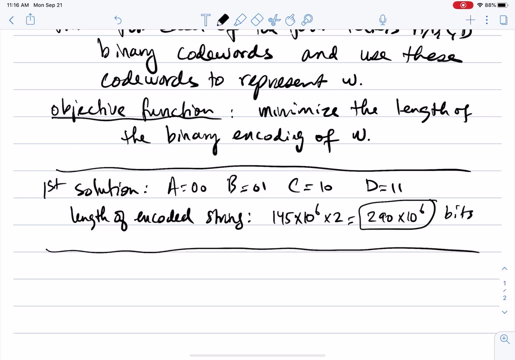 is replaced by two bits. so now it's times two, it becomes 290 million bits. okay, can we do better than that? can I represent a and B and C and D using a different, different code words? the answer is: the answer has to do with what are the frequencies of a and B and C and D and W? okay, so remember that the length 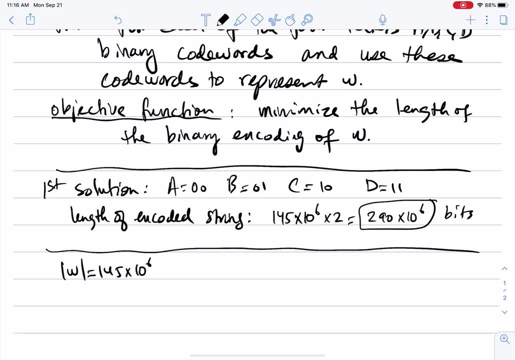 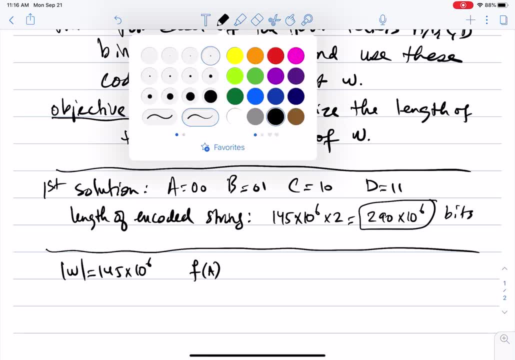 of W is 145 million. let's imagine that the frequency of a or the count of a, how many times instead of a frequency? that? just so that we don't confuse them, let me actually look at the count of a. how many times does a appear in this letter? 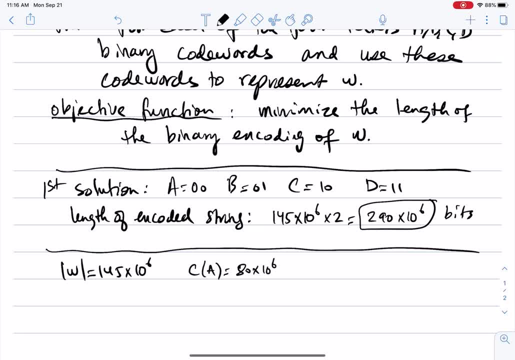 imagine it appears 80 million times. what's the count of B? let's imagine that the count of B is 20 million times. what's the count of C? imagine that it is 40 million times. so what we have here? 140 already. so let's. 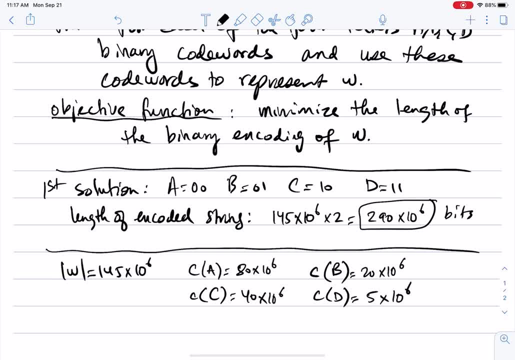 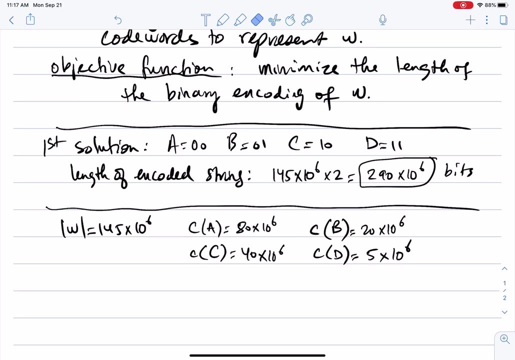 get D 5. so now we see that the four letters are not distributed uniformly. it's not appearing with equal frequencies there, so we have a to be, a is the most frequent, C is the second most frequent, B is the third most and D is the least frequent. so maybe we can do better than 290 million bits by giving. 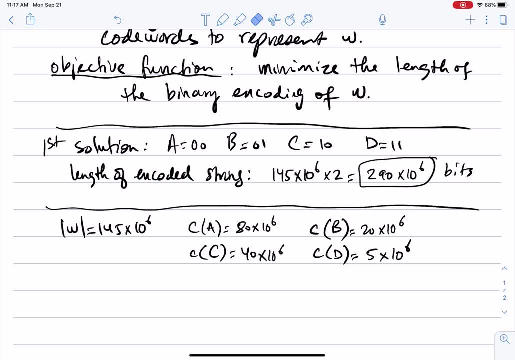 very. we're giving very short sources where greedy starts kicking in here. let's look at the most frequent letter and give it the shortest possible code word. go to the second most frequent letter, give it the second shortest possible code, and so on. so, for example, given this, since a is the most frequent, 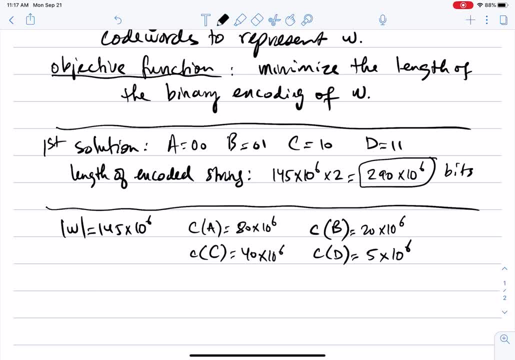 let me code word for a. I can choose the code word for a to be one one bit right. it's is the shortest possible code word I can give for a. C is the second most frequent. let me give it another short, the second shortest keyword: a code word which is: 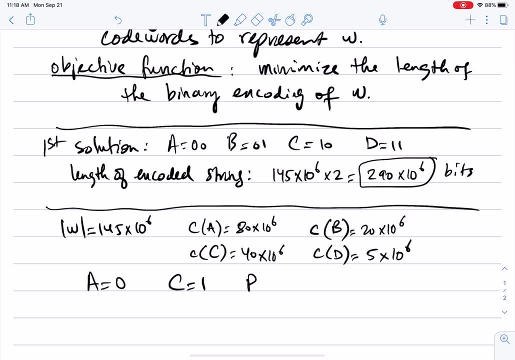 just one bit now I go to. B is the third most frequent. I ran out of code words of length one, so I can go to code words of length two. I can give B two bits and I can go to C and D and D, and now I have one. let's say that I can give it the 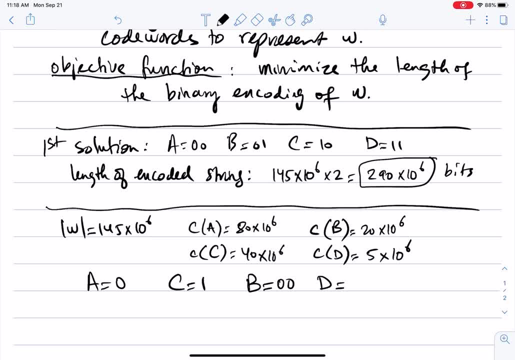 least frequent. I can give it also code word of length two, let's say zero two. okay, so this is a greedy algorithm. sort the letters in increasing order, in decreasing order of their frequency, and go through these letters based on this order. give them the shortest possible code available. okay, so at the beginning. 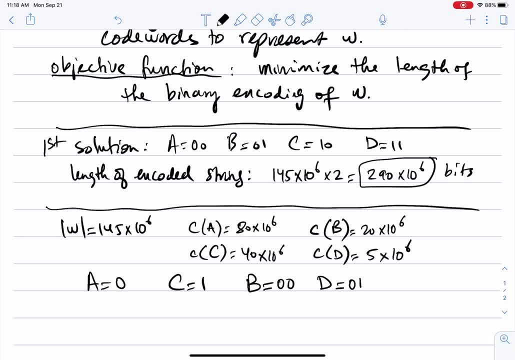 we have zero available, then we go to one, then we go to zero zero, then zero one. if, for example, the letter E was there and its frequency was equal to zero, zero so is 2 million, then E takes the code word 1, 1.. If we had F, that frequency has 1 million. 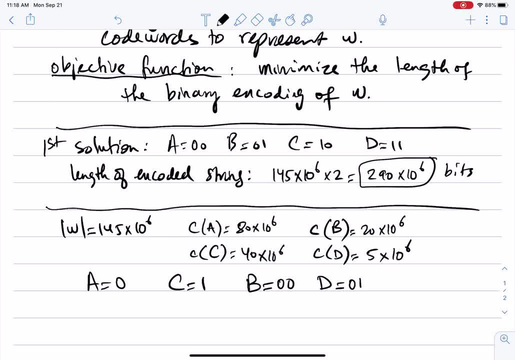 then its code word for F is 1, 0,, for example, or 1, 1.. But once we have A, B, C, D, E, F and we have, for example, the letter G that appears 500,000 times, then G now has to have. 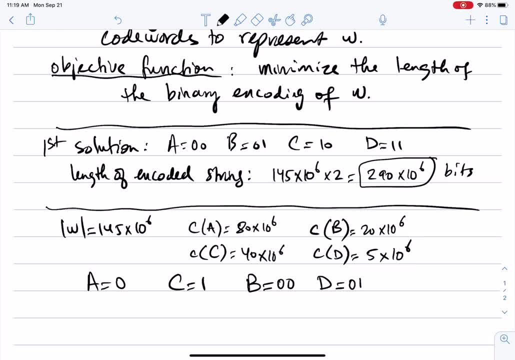 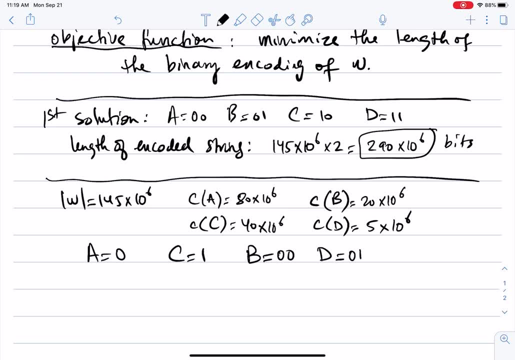 a code word of length 3, 0,, 0, 0, and so on. So this now, if I look at this, what would be the length of the encoding? So now A appears 80 million times 80 million times, and the length. 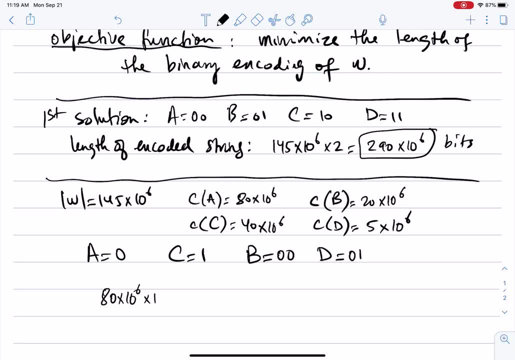 of its code word is 1.. Each one of these times is going to be encoded by one letter. This is 80 million. C is sorry, C is 40 million times. And also its length is 1.. Its code word is 1.. Okay, so this is the code word. the length Now B is 20 million times. 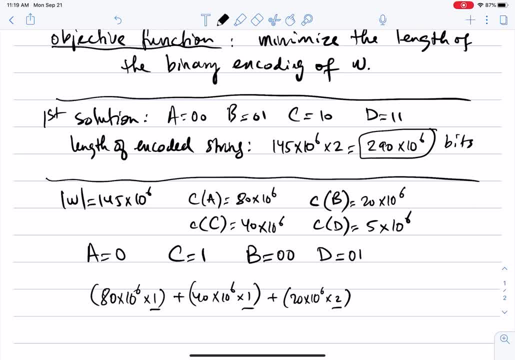 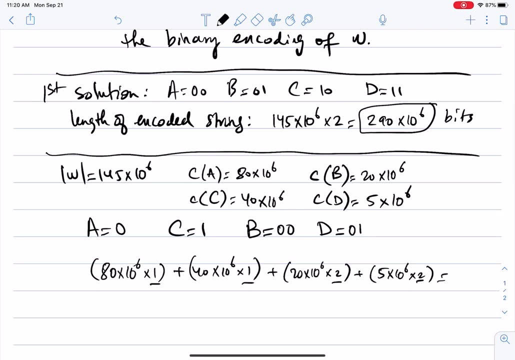 but it's now 2 bits for its code word, And what we have now, D is 5 million, but each one of them is going to be replaced by 2 bits, So now we have 80 million plus 40 million plus 40 million. 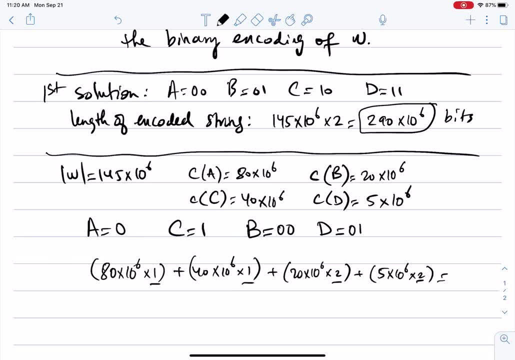 Plus 10 million here. Okay, so we added: basically the number of bits is we had what, 145, and now we added 5 and 20,, 170 million. So now we went to 170 million bits. 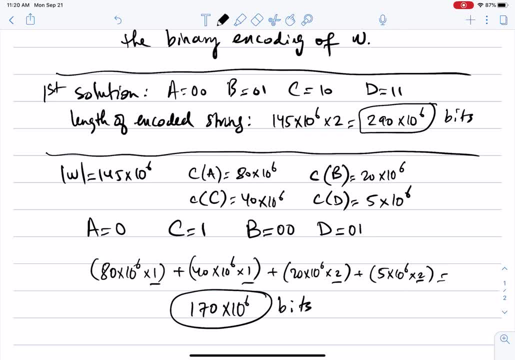 Okay. so we now encode the whole thing in 170 million bits, which is much better than 290 million bits. So now we can say: okay, this is much better. Why don't we go with this? I hope you immediately see what the problem is. because encoding is one direction, but we need to decode, right. So 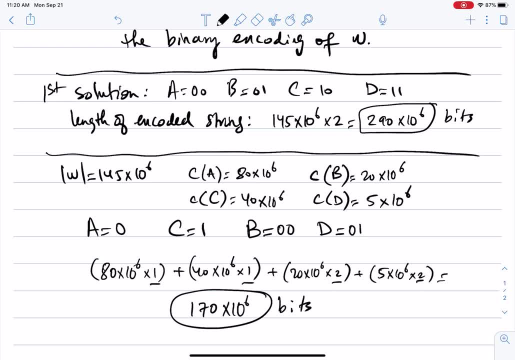 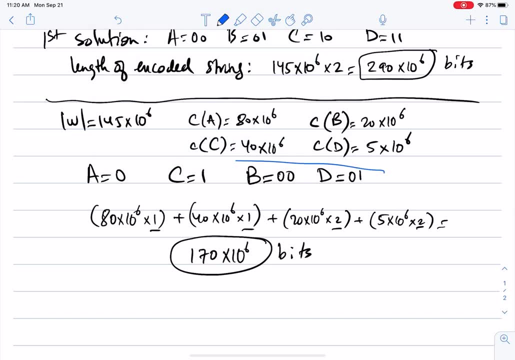 someone gives you a binary string and say: can you decode it back for me? What do you do? So imagine that under this encoding. so imagine under this encoding here. someone gives you the binary string- let's say 0001, and say: can you decode? 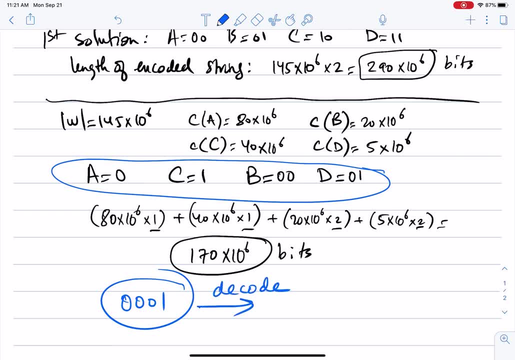 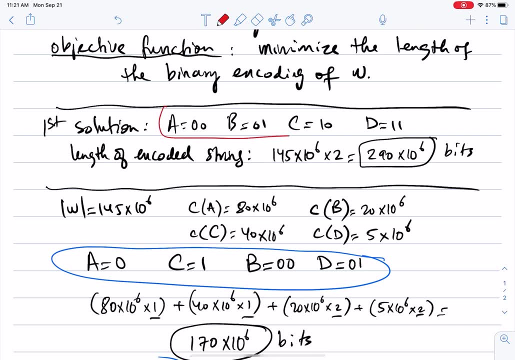 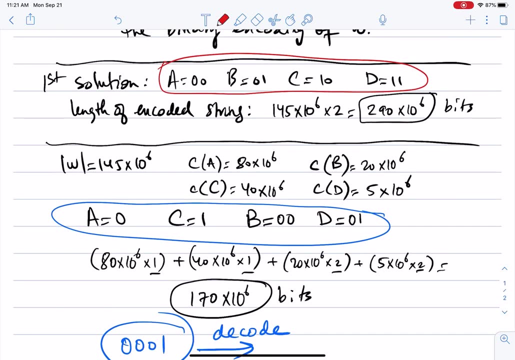 Can you tell me what this string is Under the fixed one, under the fixed one here. so we have this. all of them of length 2, 0001 has to be decoded. the 00 is A, the 01 is B, So under that, this is. 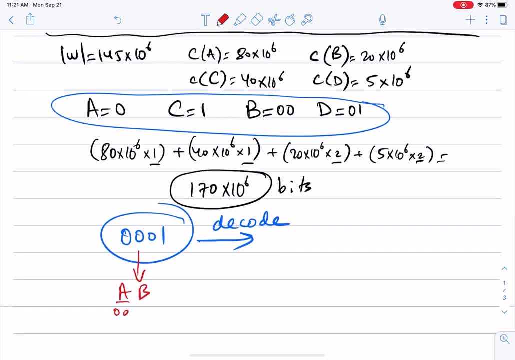 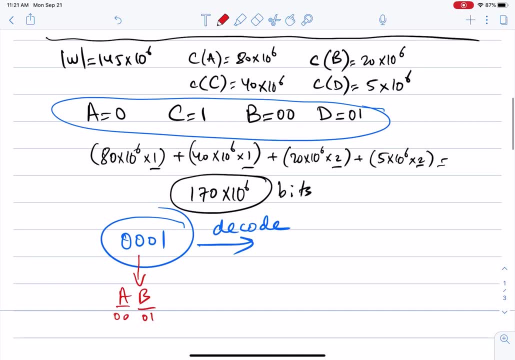 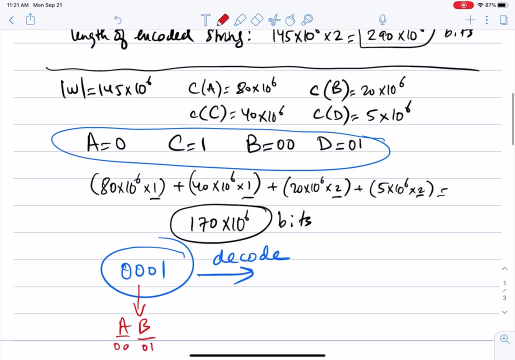 AB right, Because the A is 00, and the B is 01.. So decoding is unique, well-defined and it's and we can decode it back. We get AB. So 0001 is AB under this encoding, But what about this new one here? Well, now we run. 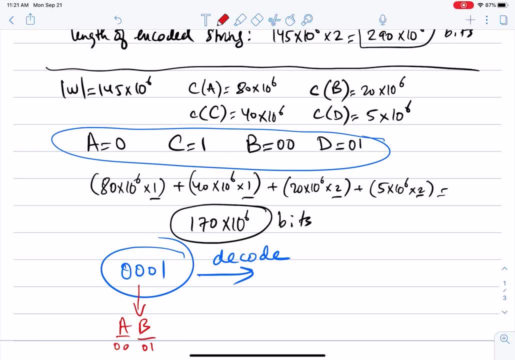 into a problem because 0001 can be treated as A, A, A C. This is one possibility I can. each one of the zeros is an A and one is a C. Another possibility is I can look at the 00 as B. 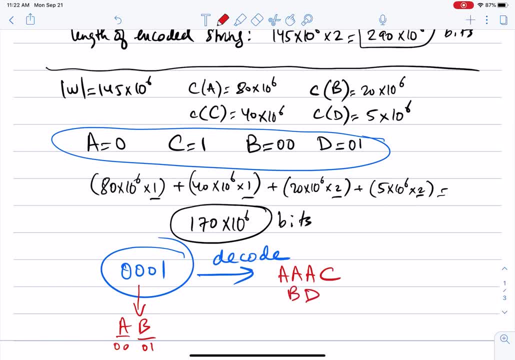 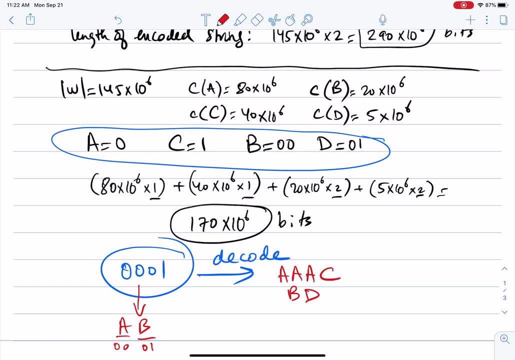 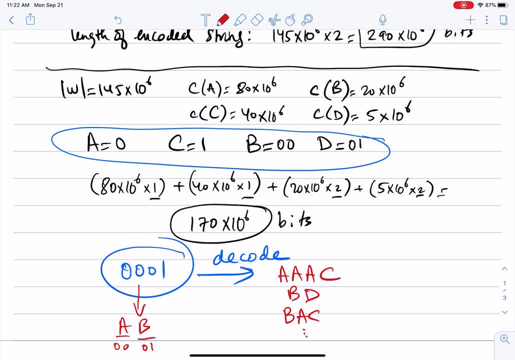 and so on. So now you see the problem that, yes, I got a shorter representation or binary encoding of W under this variable length, variable length code word, But the problem is that decoding becomes a problem. I cannot decode this uniquely, And this is where Hoffman coding comes into the 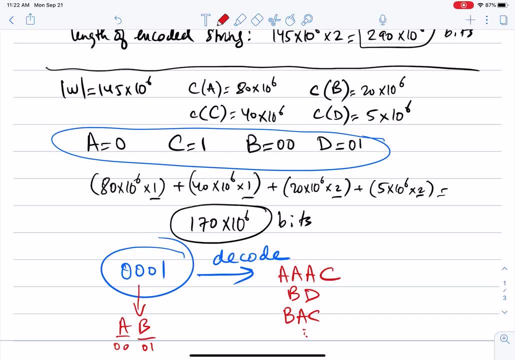 picture. Hoffman coding is a problem, And this is where Hoffman coding comes into the picture. Hoffman coding is about giving variable length code words. We don't want to give the same code word to all the letters. We want to give them code words according to their frequencies, But also. 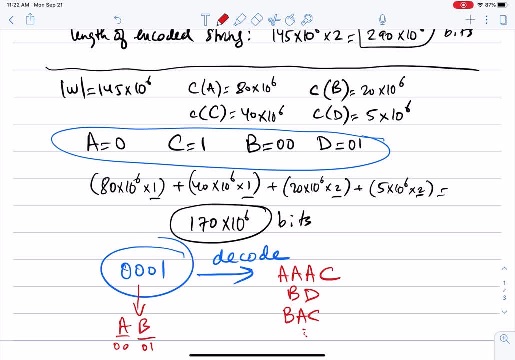 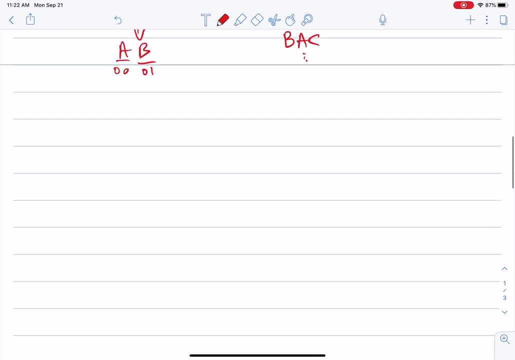 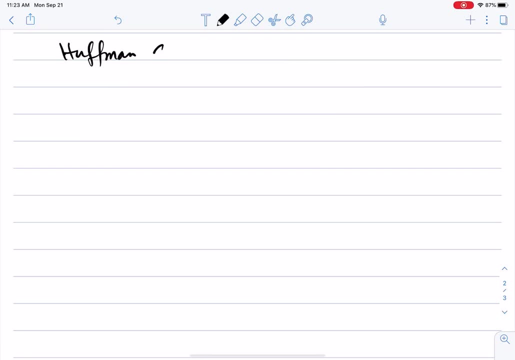 we want the decoding to be unique, Going from the binary string to the letters. we want that to be unique. So the way Hoffman coding works is the basic assumption of Hoffman coding- So now we go to Hoffman coding- Is that it is about variable length, variable length, code words. In other words, we don't have 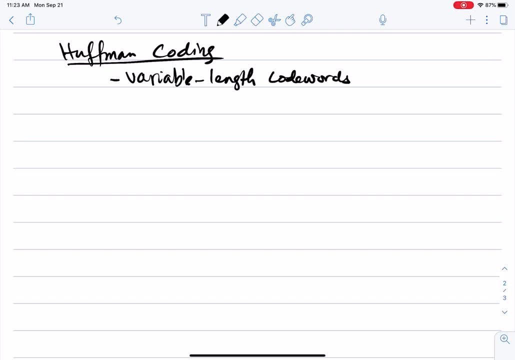 to have the same length for all binary representations of all letters. A can be two bits and D can be 15 bits. This is what I mean by variable length. The second thing, which is the most important constraint or feasibility constraint that is put: 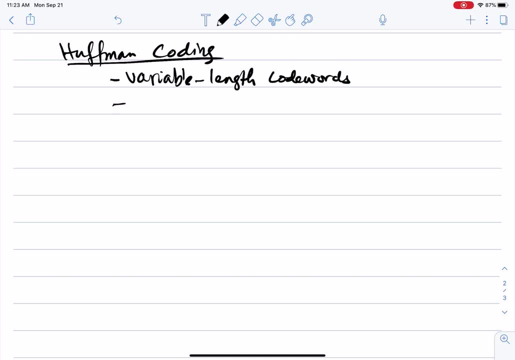 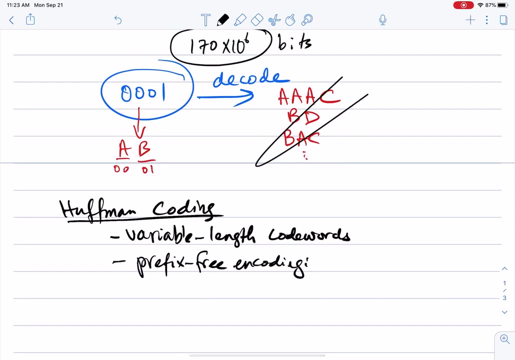 by Hoffman. coding is the notion of prefix-free encoding, Prefix-free encoding. If you think about the previous one here. what was the issue with this? Why were we getting three possible decodings here? Because we can look at 0, 0,, 0, 1, and we can say, well, maybe this is three A's. 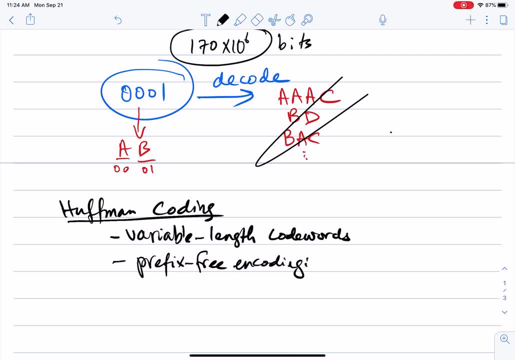 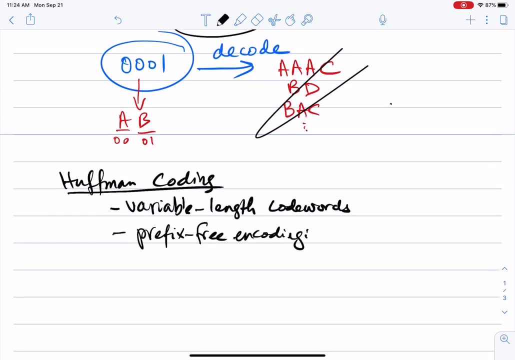 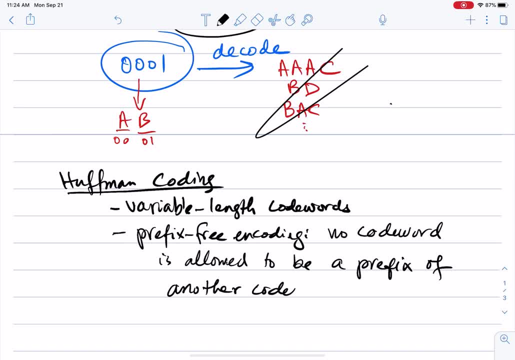 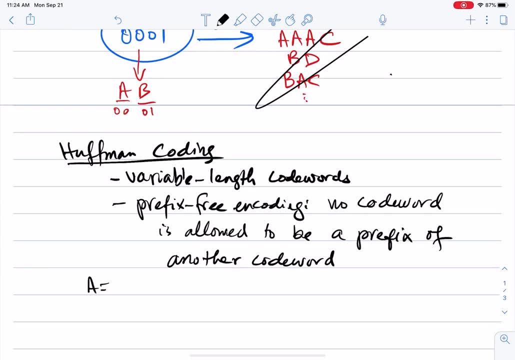 code word. another code word. Okay, So if you look at this coding here, A is 0, C. let's look at it again: If A is 0, C is 1, B is 0, 1,. 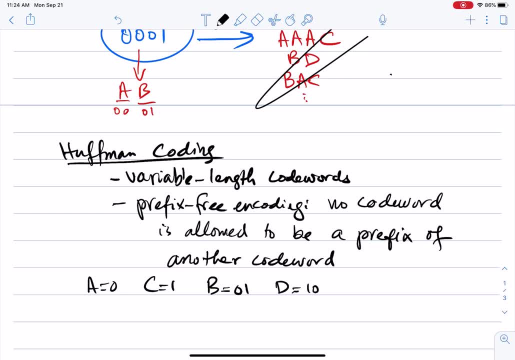 and D is 1, 0,. this is a problem here, because A is a prefix of B, A, 0 is a prefix of 0, 1.. C is a prefix of D. Okay, So this is not allowed under Hoffman coding. We don't allow something. 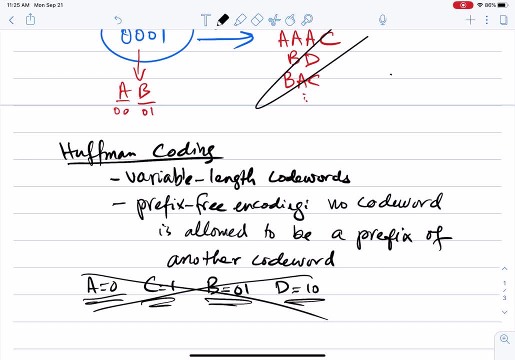 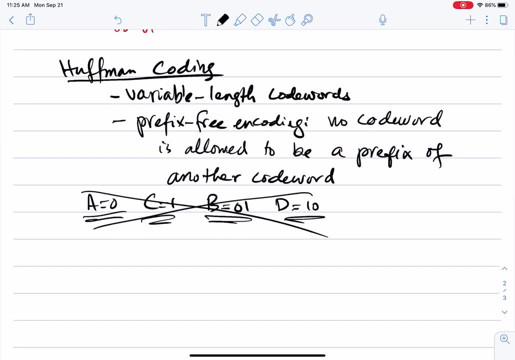 like this. So now we want to give, we want to give the, the symbols, different codes with different length, but not to our, our prefix. So you know, one example- let's say an example is- A can be 0. When A is 0, it means that the other three letters- 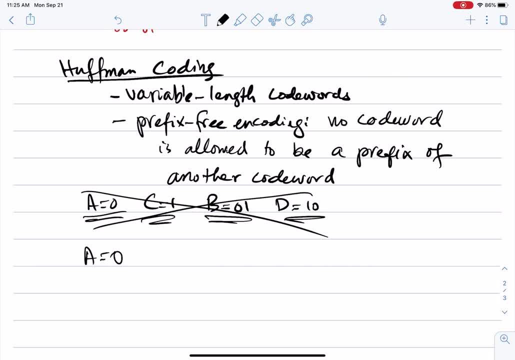 cannot start with 0, because if they start with 0, A will be a prefix. So now B has to start with 1, C has to start with 1, D has to start with 1.. But now we need to distinguish them. C, we said C. 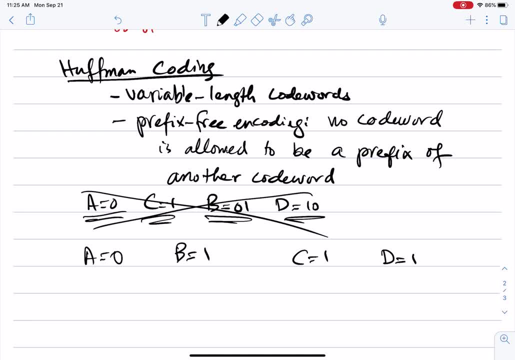 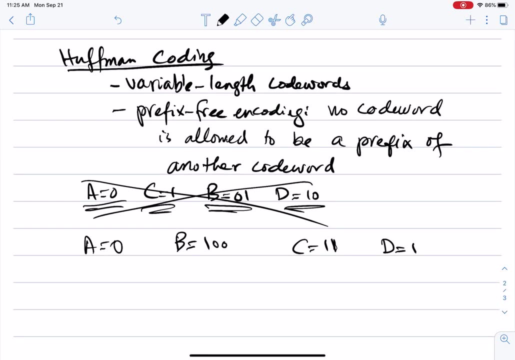 for example, is the? which one? C was the the second most frequent. so imagine that I give: C is 1, 1 here And B which one was them? B is the third most frequent. Imagine that B is 1, 0, 0, and D is 1, 0, 1.. So if you look at these three, 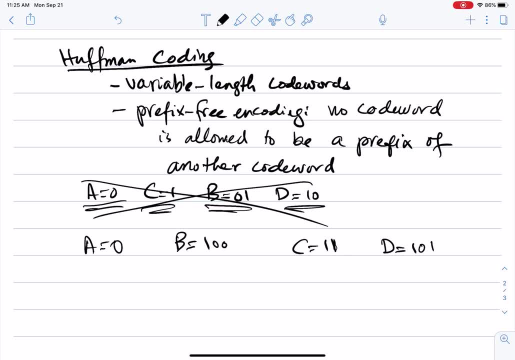 here now. A is not the prefix of any of the three. B is not the prefix of any of the three. C is not the prefix of any of the other three. D is not the prefix of any of three. So this would be a fine. 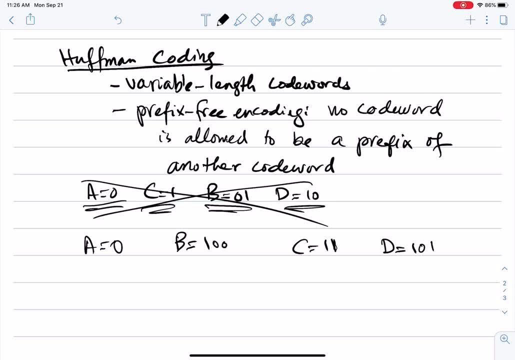 code that's variable length and none of the code words is a prefix of the other. But now we need to go back to our original problem, that we want the encoding, the encoding of W, to be the shortest possible. okay, So now we want that if I have the count for every letter, so I have the count for A. 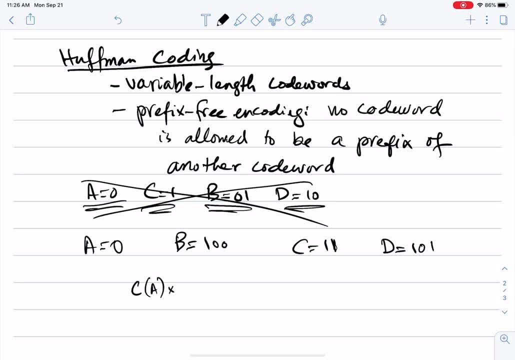 and count of B. so I want the count of A times the length of the code for A. Let's say, for example, the code for A. let's say alpha A. So alpha of A is the code, the number of bits in the encoding. 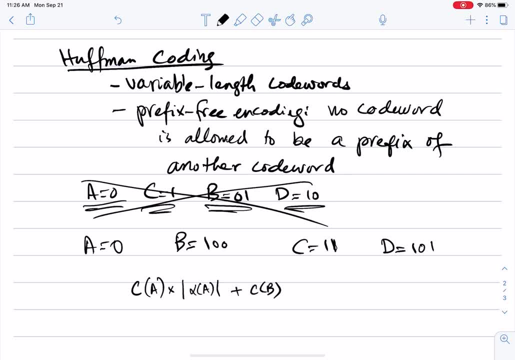 of A- We want this- plus C of B times the length of the encoding of B, plus the count of C times the length of the encoding of C, plus the count of D times the length of the encoding of D. We want this, this value, to be minimum. 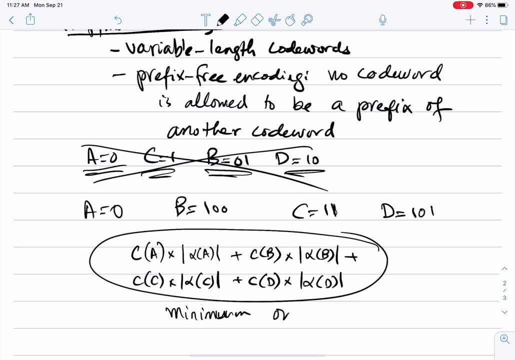 minimum over all encodings. alpha: okay, So if you come up with a different alpha, you know A is 0, 0, and B is 1, 1, 1, and so on. we want this value to be the smallest, So this is the optimality. 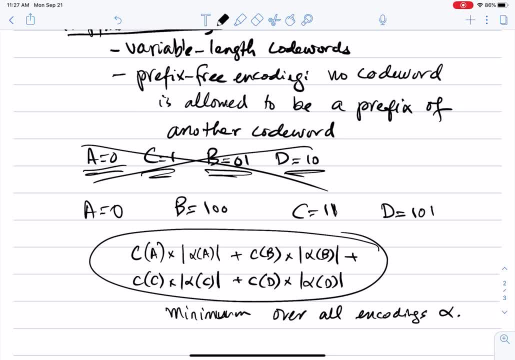 function in in that Huffman coding goes after: okay, So it wants to find binary codes for the letters and the binary codes can be of different lengths. but then when we turn that or the, the, the input string, into a binary string, 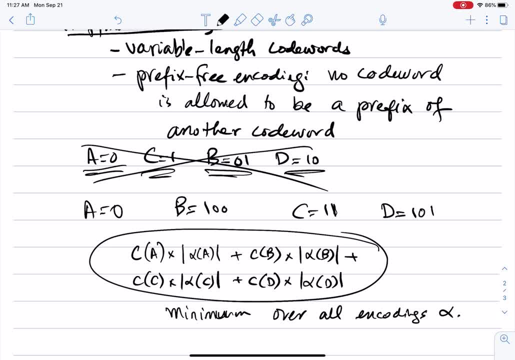 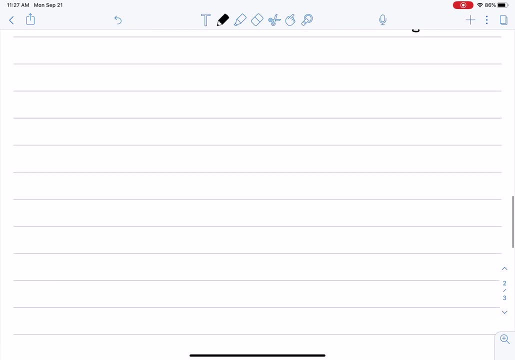 under this encoding, we want the resulting binary string to be of the shortest possible length. okay, So how does what is the, the, the binary or, sorry, the greedy algorithm for Huffman? It's the following: So Huffman encoding algorithm works as as follows: So in the first step, it creates a binary code for A, and then it creates a binary code for B, and then it creates a binary code for C, and then it creates a binary code for D, and then it creates the binary code for S, and then it creates the binary code for V. 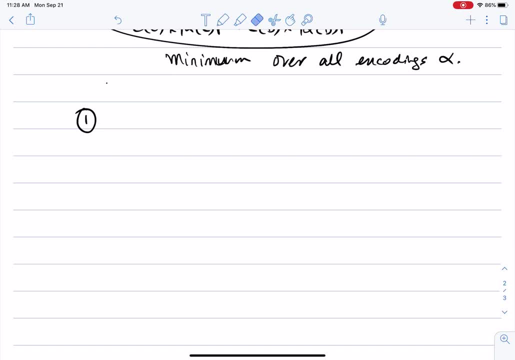 So again, imagine here the input. sorry, let me actually write it a bit cleaner. So the input is N letters. so these are the letters that will appear in the alphabet in the string in my. in my example so far I have been using N equal for ABCD, but it can be any N and the. 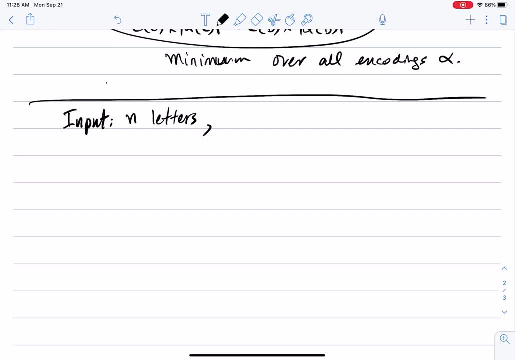 frequencies, let's call them the frequencies or counts, and frequencies which are not the correct addresses in the человека city, whenüzel, somewhat like chase frequency, which is the code of the building run in the works and in the works. 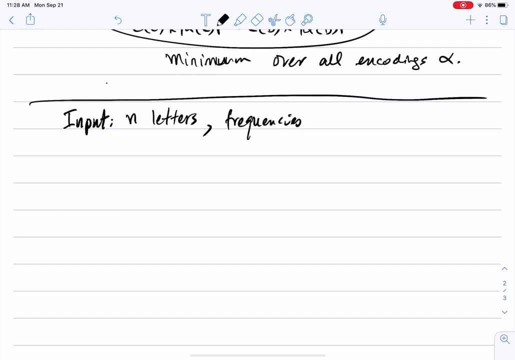 frequency, which is the code of the building run in the works and in the works frequencies of the n letters, the n. So let's F1,, F2, Fn. Okay, so F1 is the frequency of letter 1,. 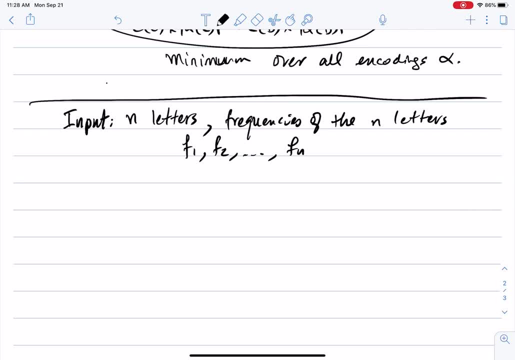 F2 is the frequency of letter 2, and so on. And remember that the and the output is code words, code words. let's call them C1, C2, to Cn, such that the sum of Ci times Fi. 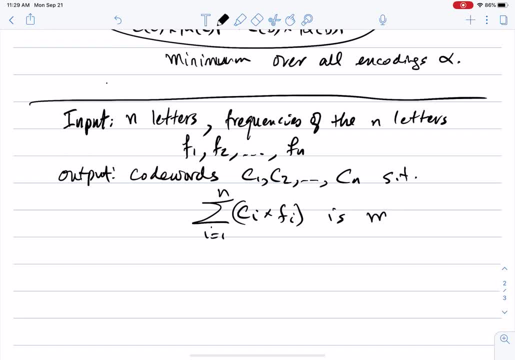 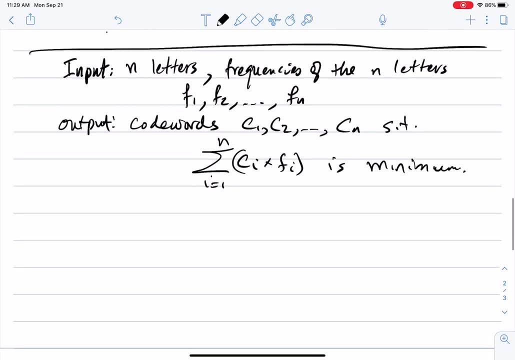 for i equal 1 to n is minimum. Okay. so if you think about it, you know how is Hoffman coding is going to work. We showed one greedy algorithm that didn't work because it caused- this problem of decoding is not unique- by saying: let's sort in. decreasing in decreasing order by the Fs. 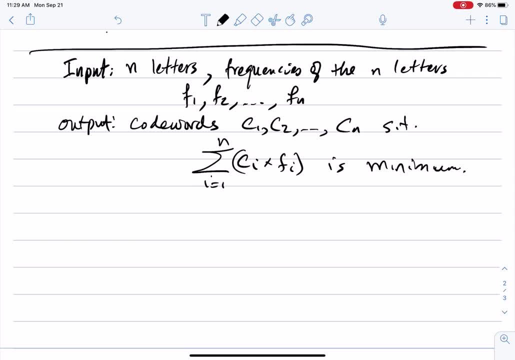 by the frequencies and assign the shortest code by that order. That is problematic. Hoffman coding does it in a smarter way that results in prefix-free code and that is optimal in terms of the value of this sum of Ci times Fi. So Hoffman coding algorithm works by first create n trees- T1,, T2, Tn- each consisting of a single node. 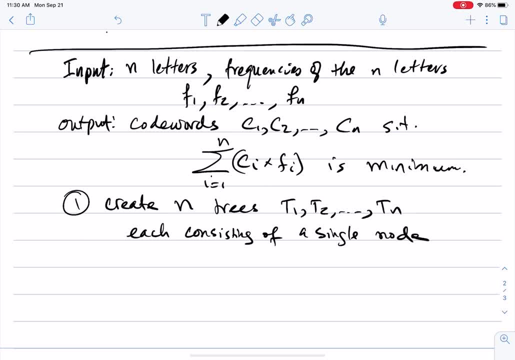 a single node and that node and the node has the sum, the frequency in of the letter for the node, for the that corresponds to that node, and the node has the frequency, and the node in tree Ti has the frequency Fi. Okay, so the algorithm will say: start by saying: 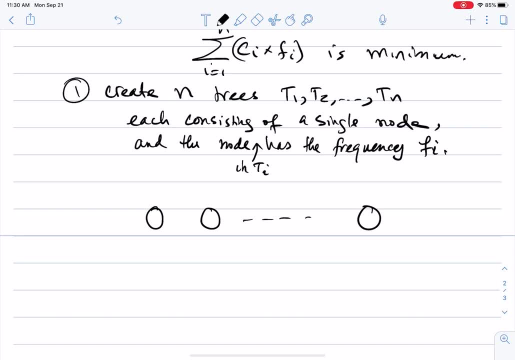 okay, let's start n trees: 1,, 2,, all the way to n, and this one here will have the frequency F1, and this one here will have the frequency F2, and this one here will have Fn. Okay, so we'll start with n trees. each one of them has exactly one node in it. 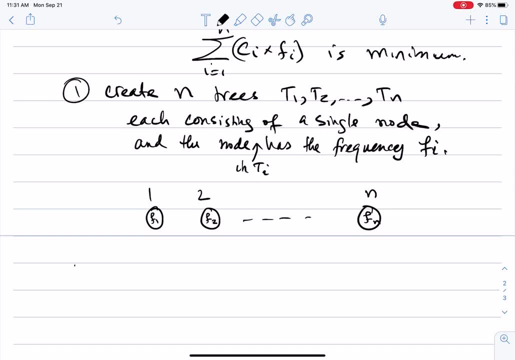 which is a root node and it has the frequency 2, we will do the following: is that repeat? Repeat the following until underneath, until we have a single tree. okay, so we are gonna start merging three trees now. okay, so we have n individual trees. we are going to merge them two at a time. okay, so we will take two. 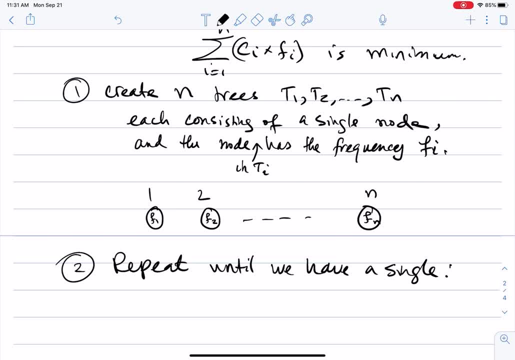 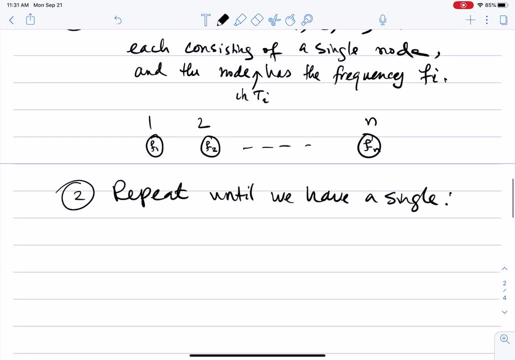 merge them. we go to n minus one trees, then we will take two, merge them, we go to n minus two trees, and so on. at the end we have one tree. okay, repeat until we have the following: find two trees, find two trees with the smallest way, with the smallest. 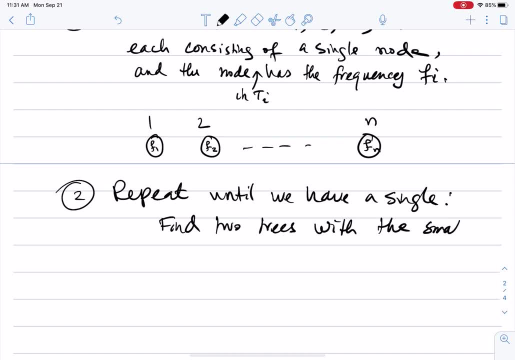 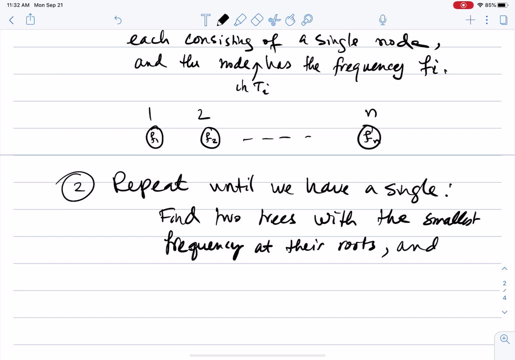 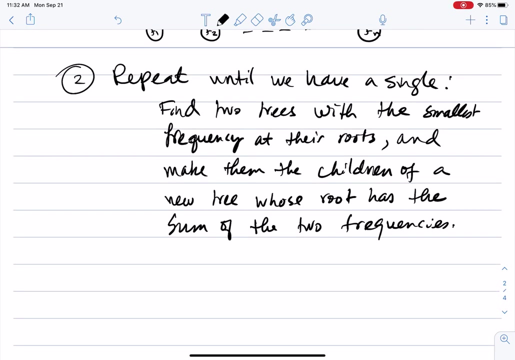 with the smallest frequency at their roots and and create and make them the children of a new tree whose the root has the sum of the two frequencies. okay, so imagine that the algorithm finds that fi, the tree that has fi and the tree that has fj- these are have the lowest. 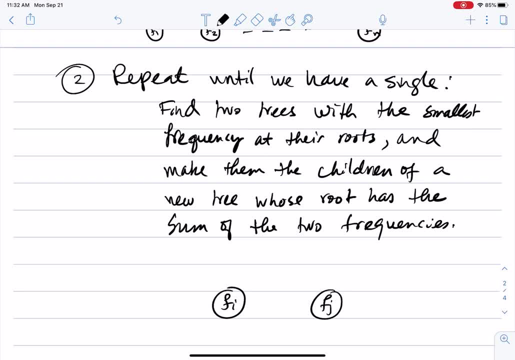 the, the smallest frequencies, okay, and now we basically take these two trees and create a new tree where, with a new root, that whose children are these trees, fi and fj, and the weight here will be fi plus fj. okay, and then we just repeat doing this, we continue doing this, okay. so let us go back to our example to illustrate this here. 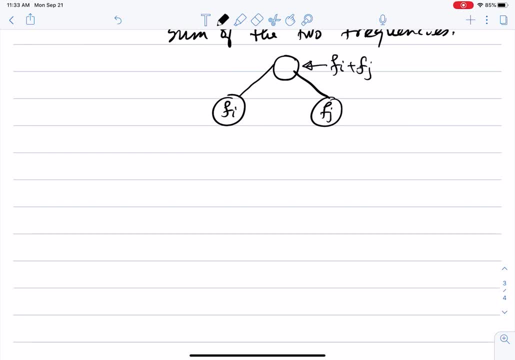 uh, so imagine that in my case, that a has frequency 0.35. okay, i want to turn things into frequencies now. b has frequency 0.1, c has frequency 0.2, d has frequency 0.2. let's say okay. so what does the 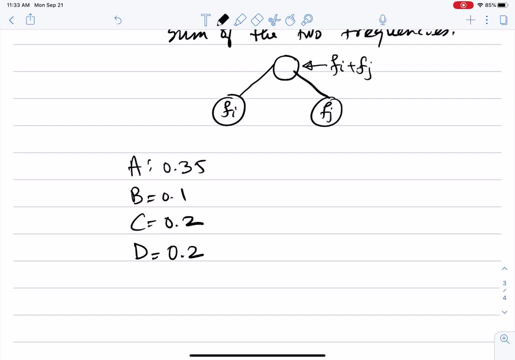 algorithm say, let's find. so the algorithm works. the first step is going to create a, a. this is the first step. in this step it says uh, c and a, quite a. this is a tree for a, a tree for b, tree for c and a tree for d, and the frequencies are going to be 0.35. 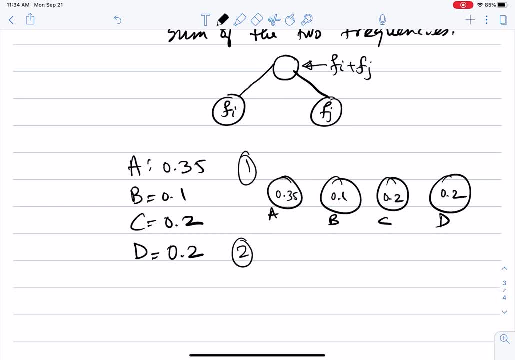 and for b 0.1, for c 0.2 and for d 0.2. so this is the first step. the second step it says: find two, no two trees in this that has the smallest values in their root. so if i look at this, that's one of them. b has to be one of them, it's the smallest. and then i need to see a physical thread, the один and meaning the name of ne denot on the line and broken index 2. this will my root, the one and working. 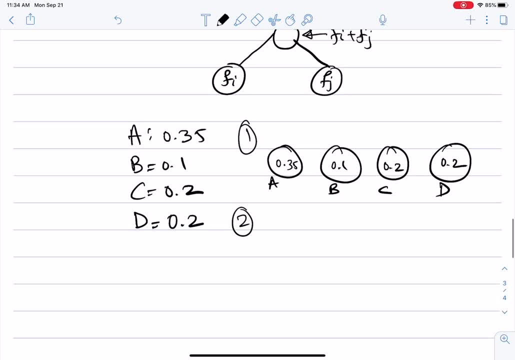 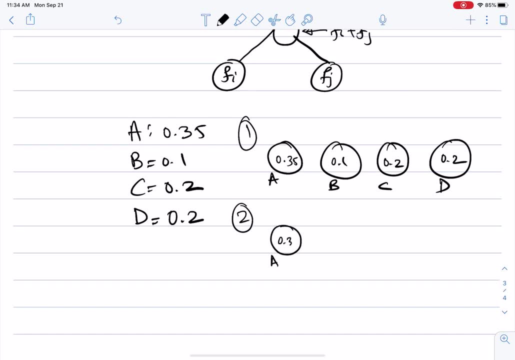 1 of them also gets the number and números n myself, and then i need to make an arbitrary choice between c and d. imagine that i take c here, so now a doesn't change, it is 0.35. now i take b, b and c and i make them as two children of that with. 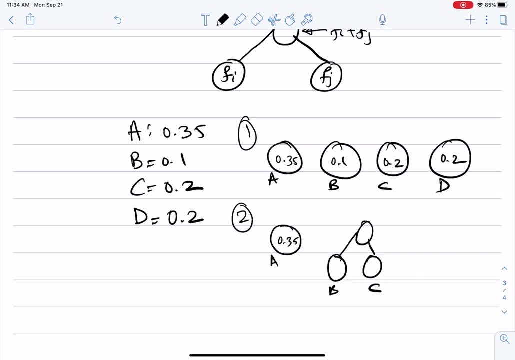 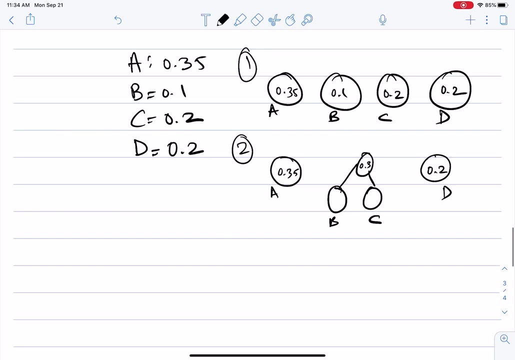 the new root, where the frequency of that new is the sum of the frequencies of b and c. so this becomes 0.3 and c and d- sorry is still there. so now we went to three trees: the tree that corresponds to a, the tree that corresponds to b and c, the tree that corresponds to d. we repeat the second, the, the. 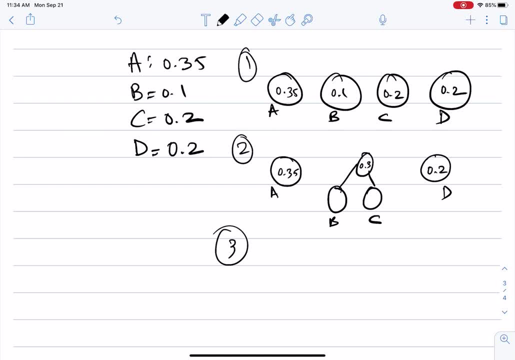 next step is: let me find, of these three trees, which two of them have the smallest frequencies. well, we find that it is: one is 0.2 and one is 0.3. and one point i didn't make there when i took b and c. it doesn't mean it doesn't matter. 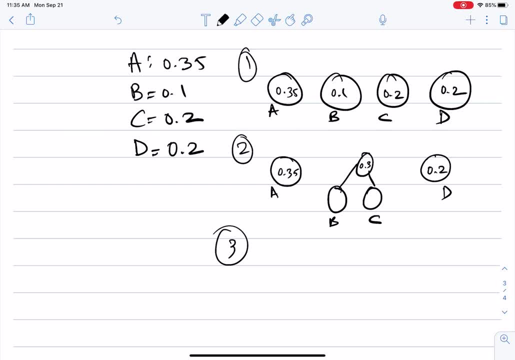 you can make b the left and see the right child, or or, uh, see their left and be the right child. okay, so now i will look at b and c, and and d. these are the two smallest, so a remains here as 0.35, as a tree by itself. and now we take b, c and d just so that i create a different. 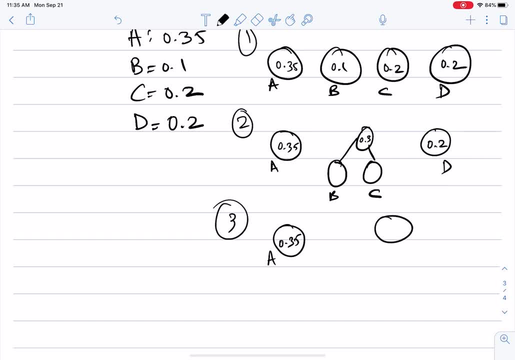 scenario here. i will make b c actually the right child. so i add that, i add this. so this is b c and this is d. so the new, the new node, the new root has a, two children: d as the left child and the other one is the tree that has b and c. so d had we know that d had 0.2 here. 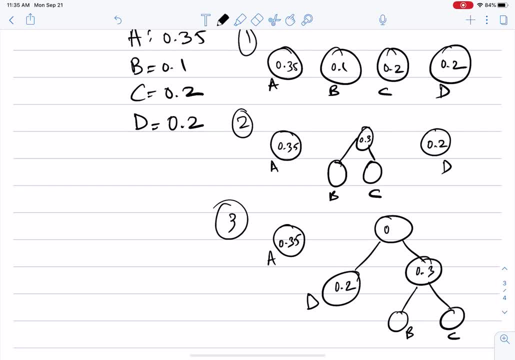 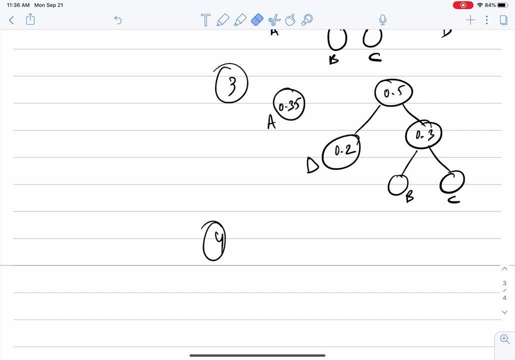 and the other one had 0.3, so this is going to have 0.5. okay, so this is what we get now. and the last step: i don't have much choice here. we create, we create a new node here whose left child is a. 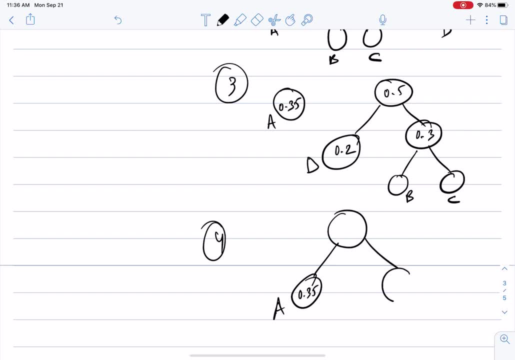 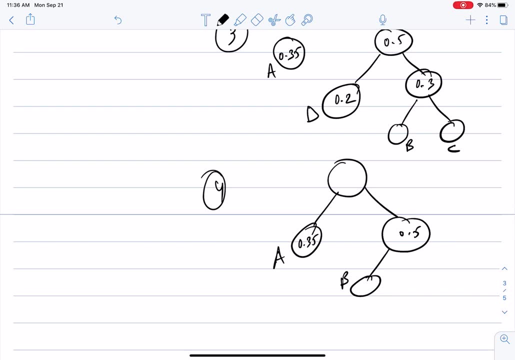 and this is 0.35. and here we have this 0.5 and b here. no, sorry, this is d and this child here is b and c. okay, so this is the the second step of of hoffman encoding and the third step of hoffman encoding. the third step is we basically give for the 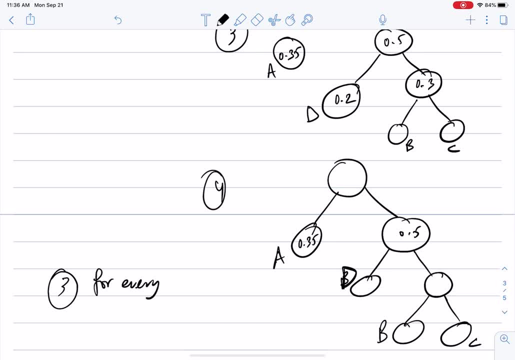 for every node. for every node, label the left edge 0 and label the right edge one. so if i do this for this tree, here i label: this is left zero, the right is one, left is zero, right is one, left is zero and right is one. and then the fourth step here. 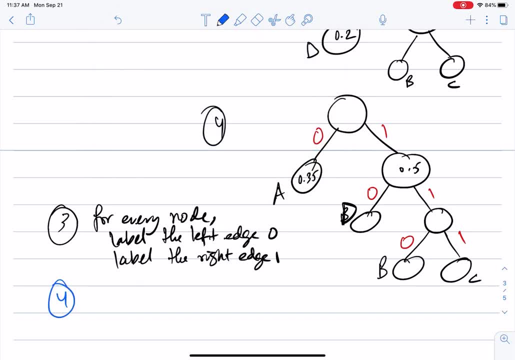 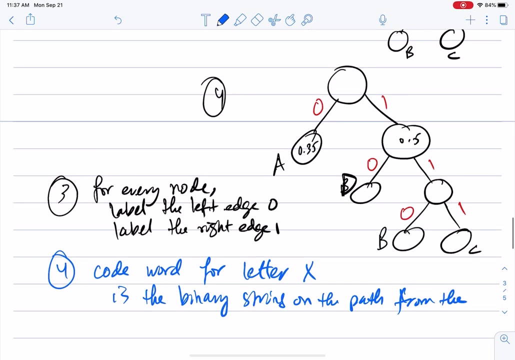 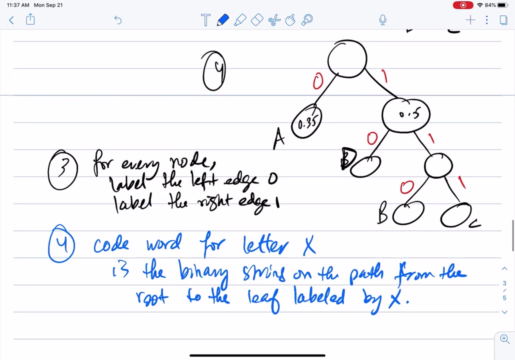 The fourth step. the code word for letter X is the binary string on the path from the root to the leaf labeled by X. Okay, so the last step now. I get the code words from this. So if you look at that tree there, for every letter you have a path from the root to the leaf that's labeled by that letter. 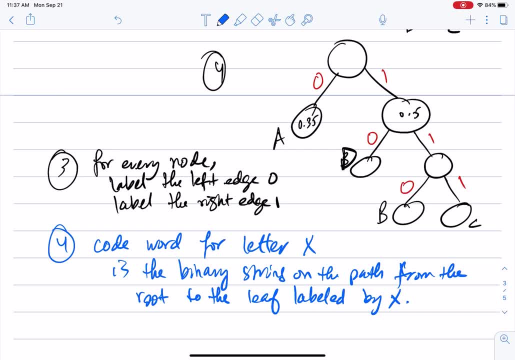 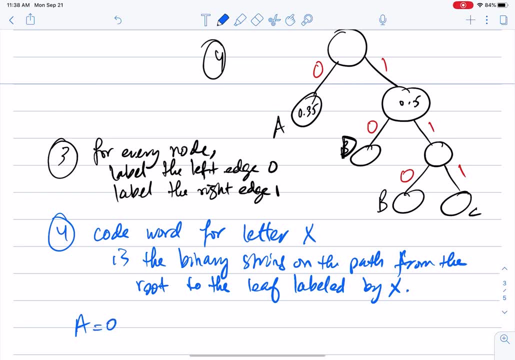 Just take the zeros and ones on that path to be the code word. So if I look at A, the path from the root to A has one edge that's labeled by zero. If I look at B, I follow the path from the root to B. 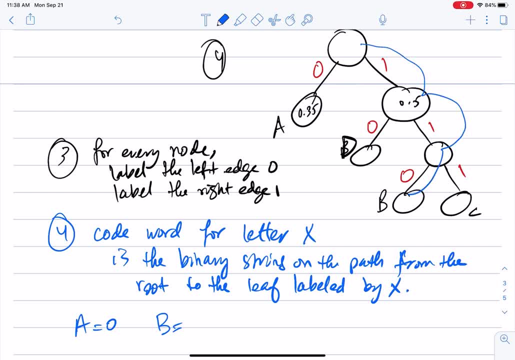 I come this way and this way I followed right, right, left, So it's one, one zero. And if I look at C, I went right, right, right, Okay. so right child from the root, then right child from the child, then right child from the grandchild to get to C. 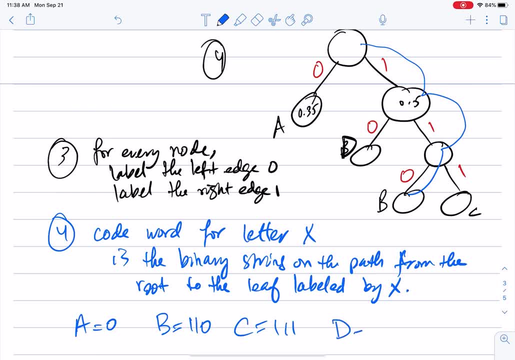 It is one, one one. If I look at D, then we go from the root to the right child and from the right child to the left child to get to D. It is one zero And this will be The code, the code words obtained by Huffman coding here. 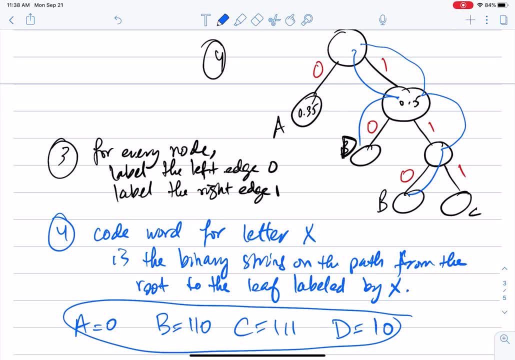 Okay, Now, if you look at these and you look at the length of original W and you encode it in the binary way according to this: that you replace A by zero, you replace B by one one zero, You replace C by one one one and D by one zero. 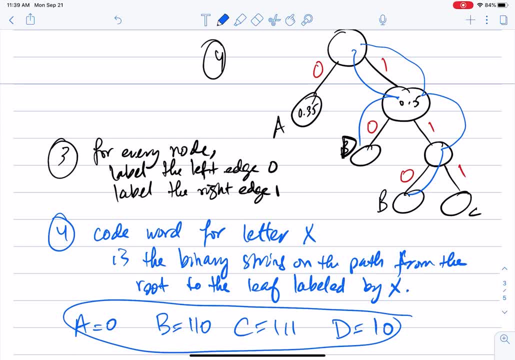 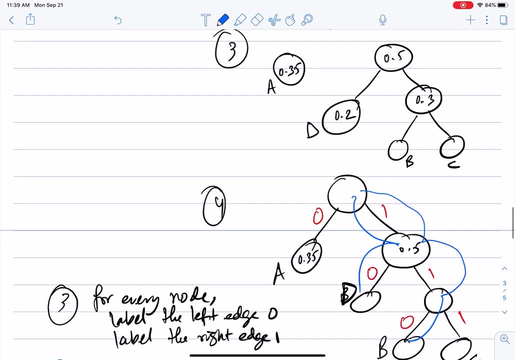 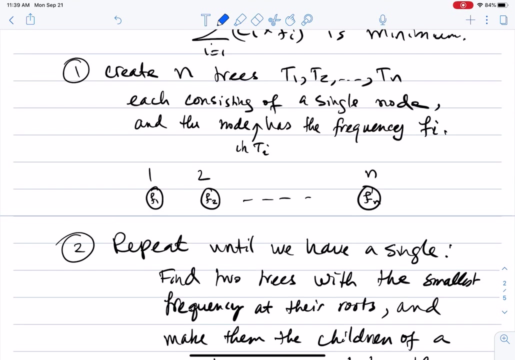 This is guaranteed to give you the shortest possible binary encoding of the original W Over all possible. And this is basically the algorithm. uh, it is greedy in the in the following sense: here, in the very first step, in the very first, in the first step, we created the trees with their weights. 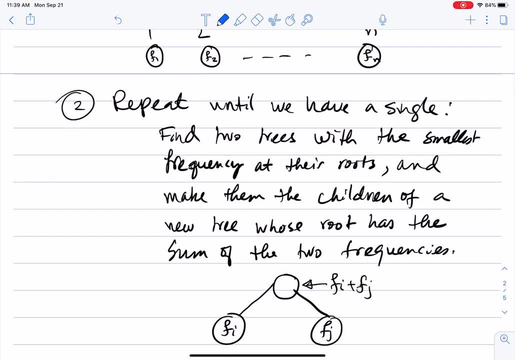 There's nothing greedy there. in the second step, This is where we make the greedy thing here. So the algorithm is working by making the least frequent letter the deepest in the tree. the least frequent letters are going to be Come the deepest in the tree. 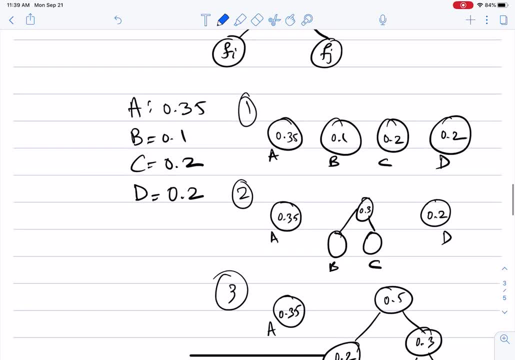 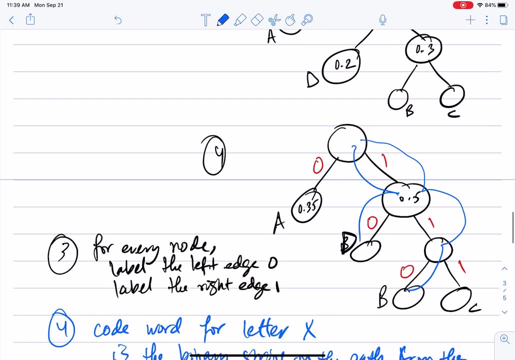 The most frequent letters are going to be the shallow West in the tree. So here, when we looked at this example, for example B was the least frequent And if you look at it in the tree it is the deepest. Okay, 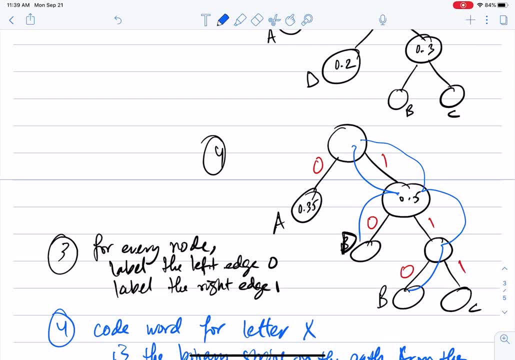 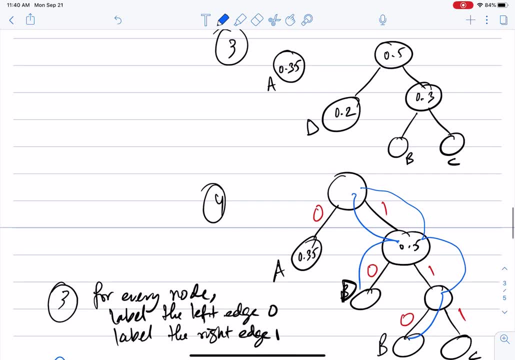 The depth of B is three. I had to take three edges to get to it. If you look at a, it's the, it's the most frequent and it is the shallowest. The depth of a is just one. Okay, And this is the greedy choice that Hoffman coding algorithm does. 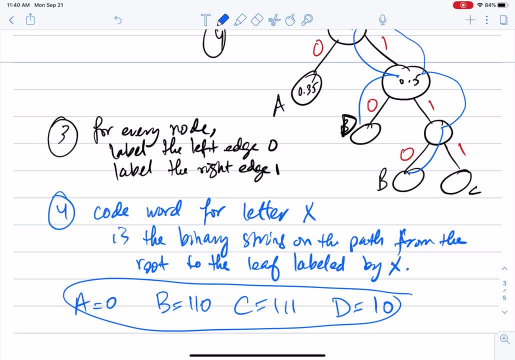 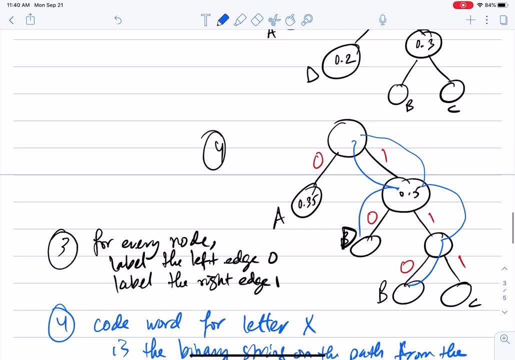 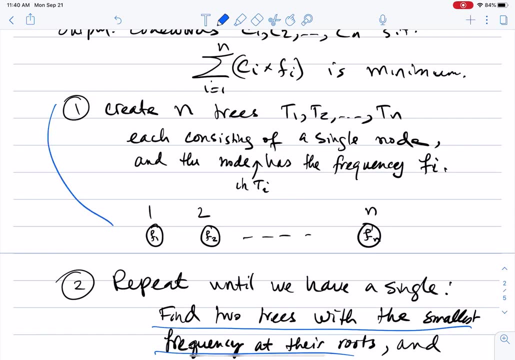 And It does it again by taking the least frequent letters, making them as a subtree, then continuing this. What's the running time of this algorithm? again, first building these trees. uh, building these trees here. This is O of N nothing fancy, right. 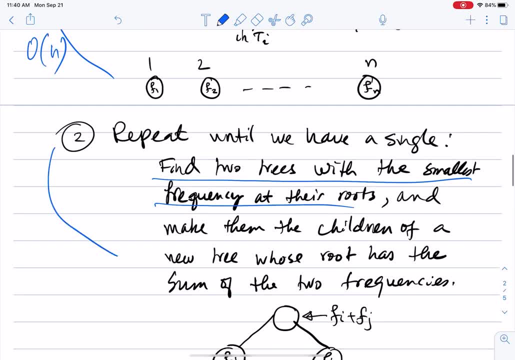 We just want to build N trees. This now will take O of N log N. N log N. If repeating this multiple times this will take us N log N. If you again use a min heap to keep the letters with their frequencies in the min heap. 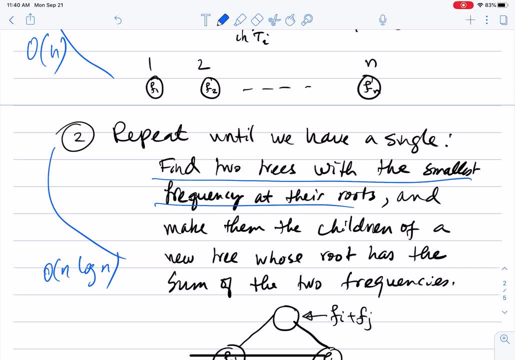 So that at the top of the heap you always have the least frequent uh letter or the root with the least frequent, the smallest frequency in it in that structure. So this is an O of N log N greedy algorithm that will produce the optimal code words: variable length code words that are prefix free for. 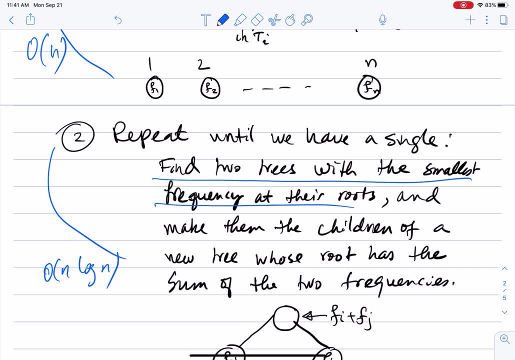 Encoding, uh, uh, any string of over N letters over N different letters into a binary string. Okay, As I said, I will not prove correctness of this algorithm, but I highly encourage you to prove the correctness of this algorithm As we talked about it before. to prove the correctness again, follow the same technique.